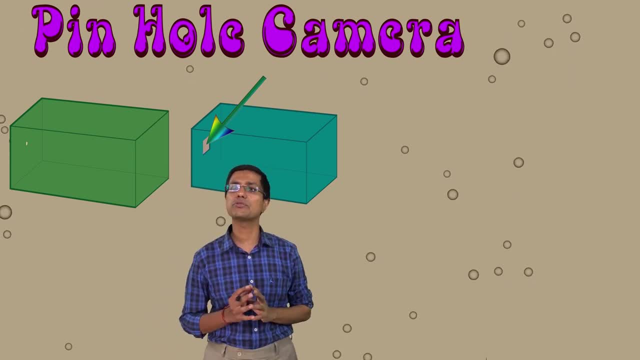 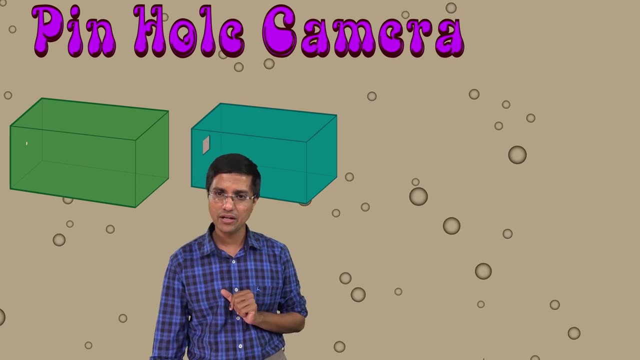 the box and then we cover it with a translucent paper. Any kind of translucent paper would do, for example, butter paper would do. okay, Tracing paper would do. So we cover this hole with a tracing paper. I put the smaller box inside. 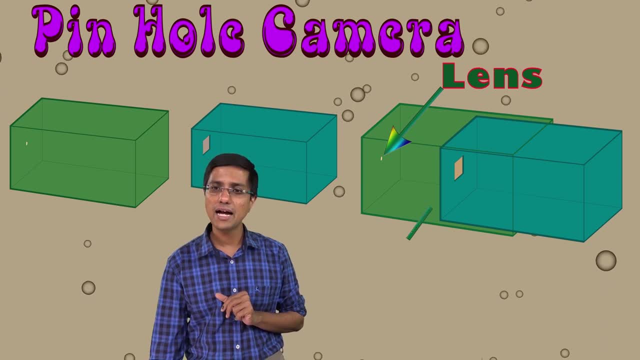 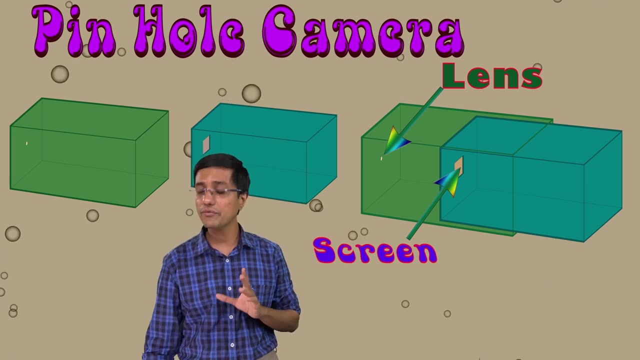 The larger one, And what would happen is that, through this pinhole, I would be able to capture the images of the world outside, and these images would then be formed on this piece of translucent paper, Something like this. So now this pinhole camera, the light rays, 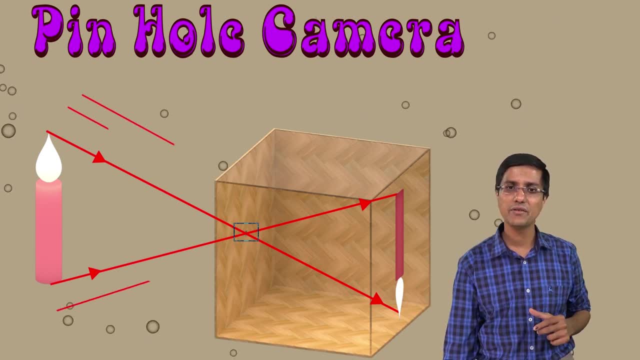 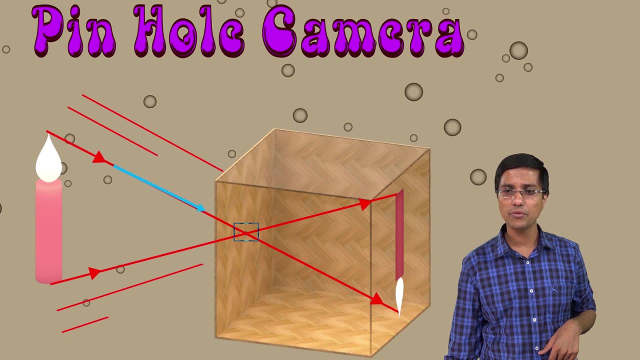 coming from the top right. The light rays, photons of light getting reflected from this tree are coming from here and of course, from here they can only go down. That is the only way they can go. So they go down From the top, they go down. 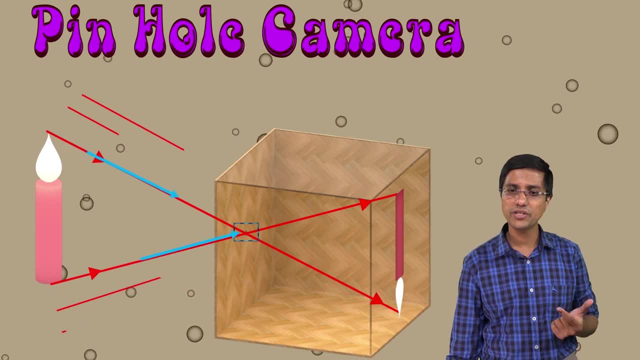 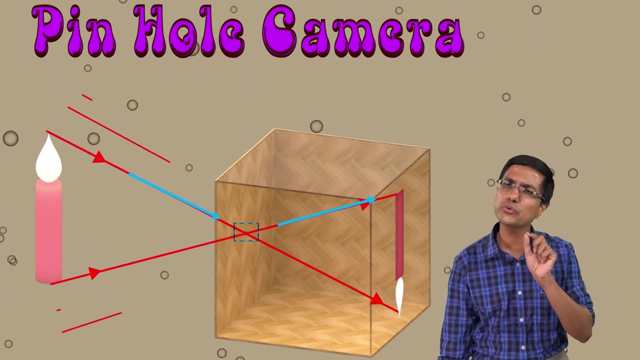 and from the bottom, the rays of light, the photons, they come, they enter this pinhole and from here they can only go up. So it masks all of it. This pinhole is so small that it stops all other photons from coming. It only allows the photons which start from. 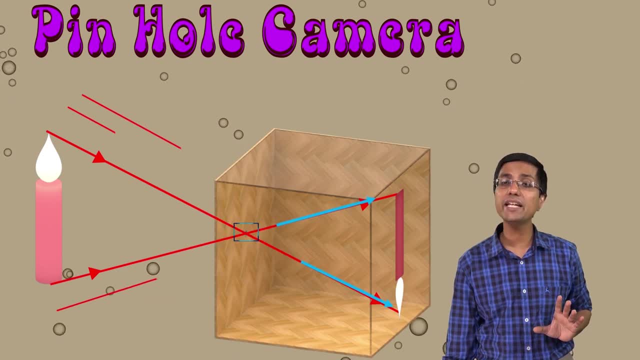 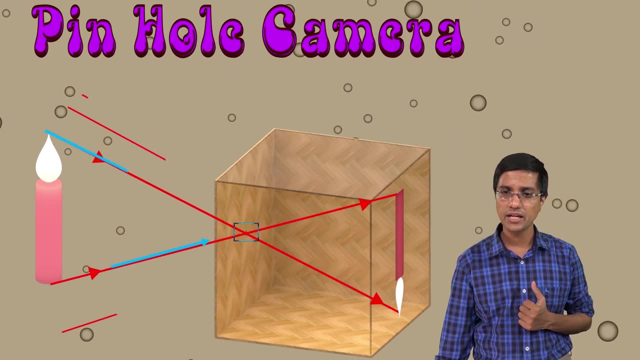 the bottom, and the only region they can go is towards the top. That is the only photons it allows. See, we already said that light has rectilinear propagation, so it always travels in a straight line Because it is blocking all other photons. 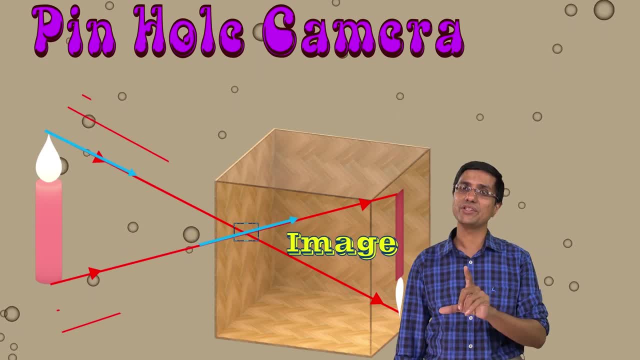 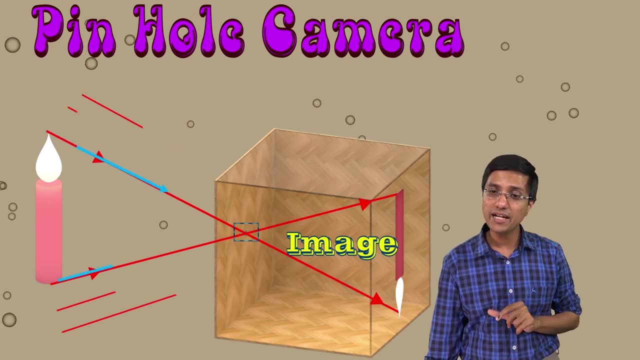 we are able to get a very clear image. Remember, it is an image, it is clear. I am able to make out exactly what is outside. so, therefore, it is an image We are able to make out. we are able to get a very clear image of whatever is outside. This image because the top photons 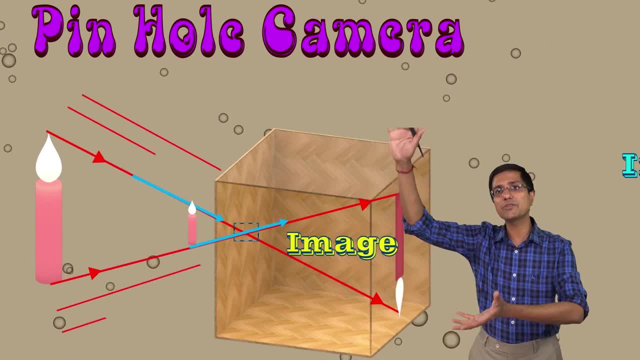 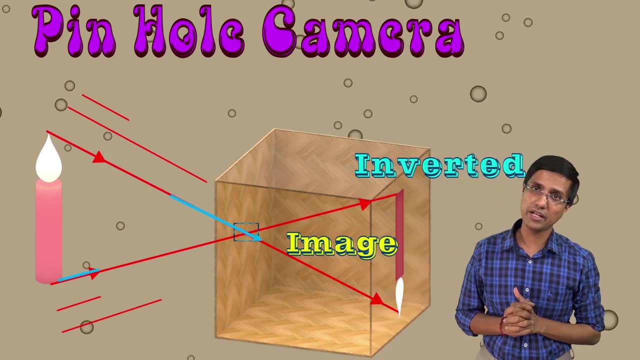 go to the bottom, the bottom photons go to the top. this image is actually inverted. So whatever is outside, I am getting an inverted thing inside. That is the property of the pinhole camera. Another property is that it does not use any lens, So the camera inside. 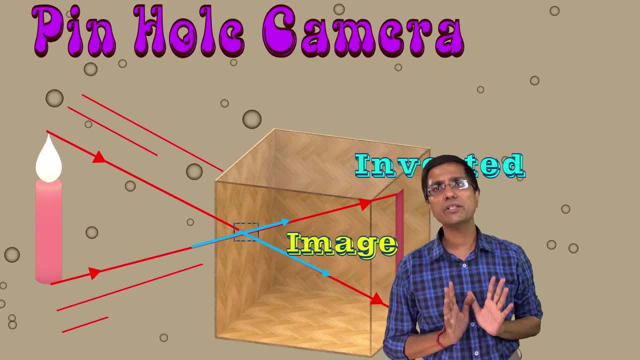 your cell phone in your camera. whatever you have does not have a lens. So the camera, cameras, digital cameras in the photography shop, all the cameras that you see, they all use lenses. This pinhole camera does not use lenses. 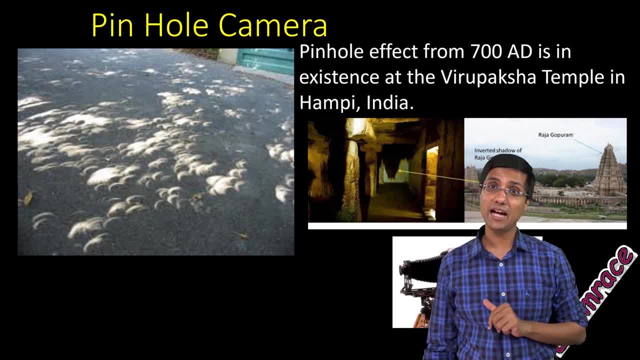 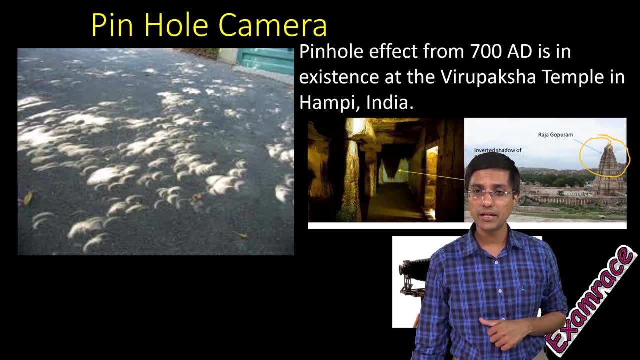 Now, of course, pinhole camera has several applications. Look, there is a temple in Hampi, India, where they have used this concept of pinhole camera and they are able to project the image of this top of the temple inside the cave on the other side.